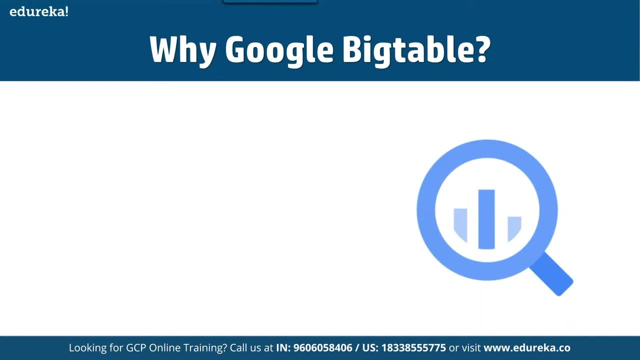 implement. It's not complicated like other vendors. It's very easy to understand and implement At the same time. by just going through the options, you can easily implement it. Plus, they have the unique data warehouse service, which makes it not only easy, but 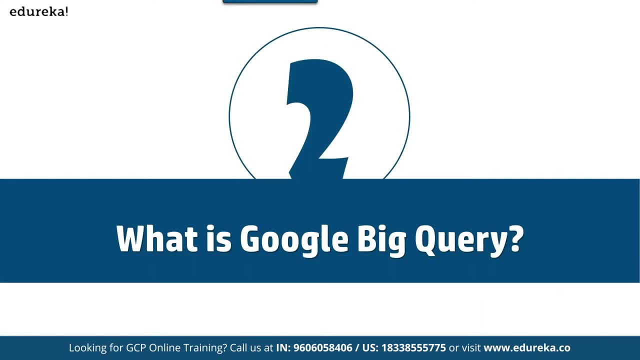 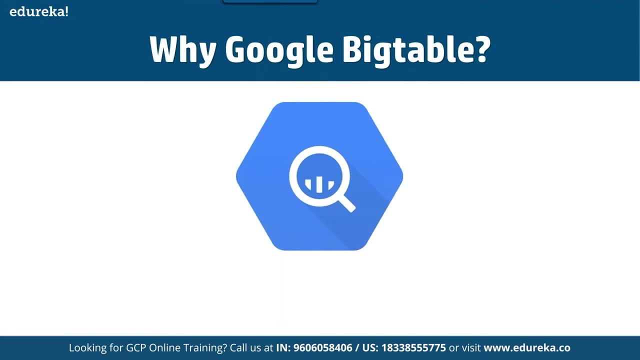 more reliable. Now, talking about what is Google BigQuery. So talking about why Google Bigtable. So your BigQuery is a fully managed serverless data warehouse which enables scalable analysis over petabytes of data. If you don't know petabytes, like you have KB, then you. 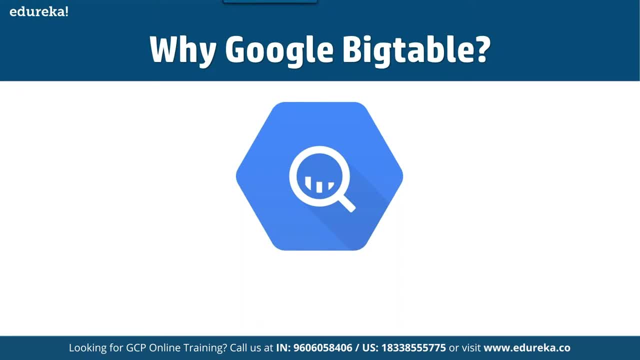 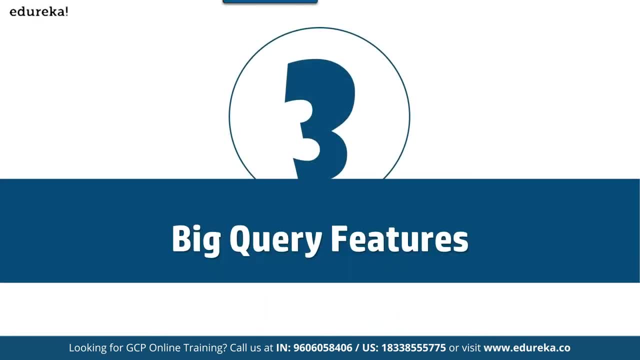 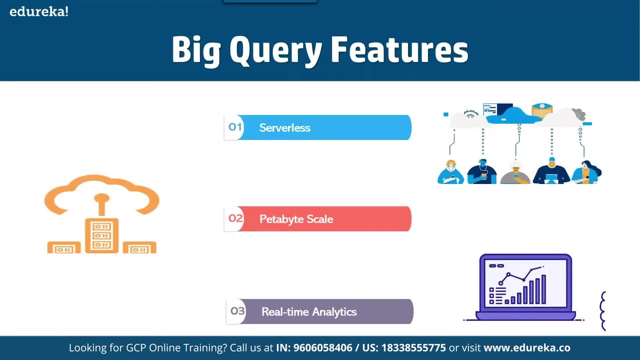 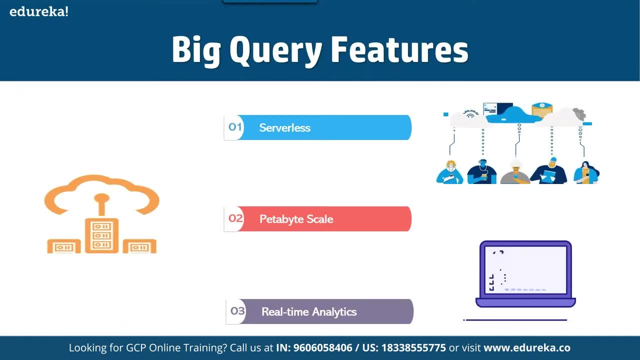 BigQuery. So very first thing is: it's a serverless, So you don't require a dedicated server. It's basically a serverless environment which is not depending on any of the hardware platform, because the entire thing services are going to be hosted on the cloud provider. 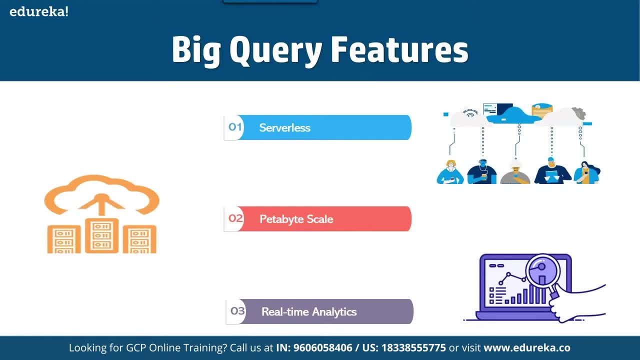 So that's why it's a serverless- one of the biggest advantage. Second, it's a petabyte to do a real-time retry, real-time analytics- all such kind of things are basically being possible with this. in addition to that, you are going to have a flexible pricing model. it's not like that. 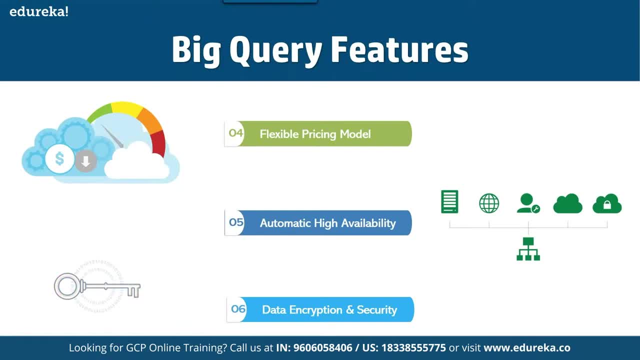 you have to take a commitment. you can use pay as you go service. so whatever you have utilized, whatever you have consumed, you are going to, you know, going to pay accordingly. according to that, next is automatic ha, which is automatic higher variability, so automatic clustering can be set. 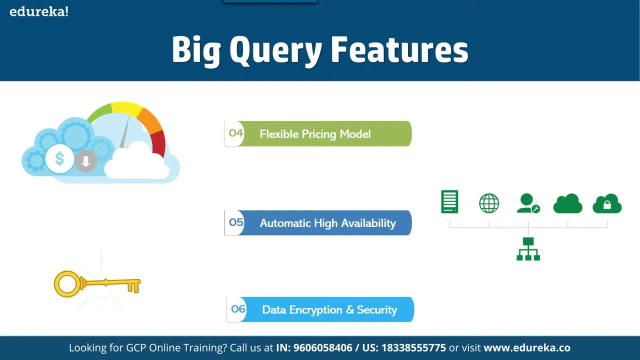 up in this case, with the help of which you can create the cluster effectively and efficiently. next is des, which is data encryption and security. now, here, in this case, there are key management solutions which are being provided, so you can have the key management solutions, security, each and. 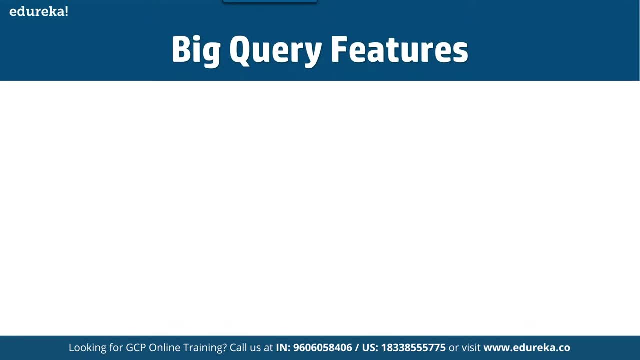 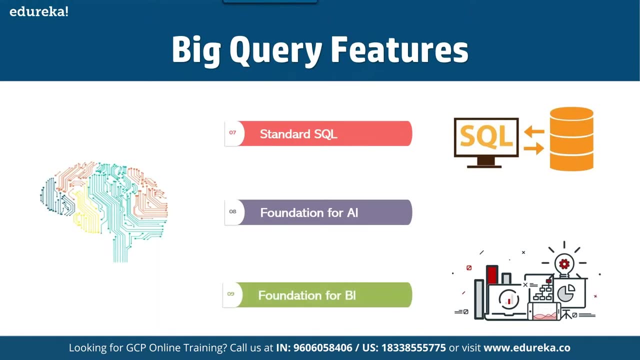 everything which is going to be provided to you at the sake of ease. now, in addition, that you are going to have the standard sql, where you are going to have the standard database which is being available with uh, you can use database as a service as well, or you can use a server on which you can. 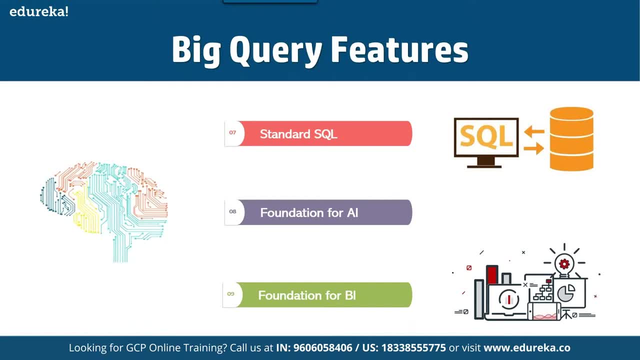 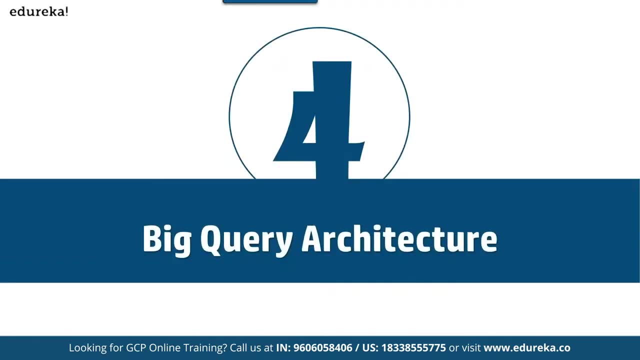 install the database. second, uh is foundations of air. so this is the foundation of your artificial intelligence and your business intelligence as well. now, talking about b, q, e, which is big query architecture, just telling you a little bit overview of it. so you're going to have the colossus, uh, wherein? uh? you are going to have 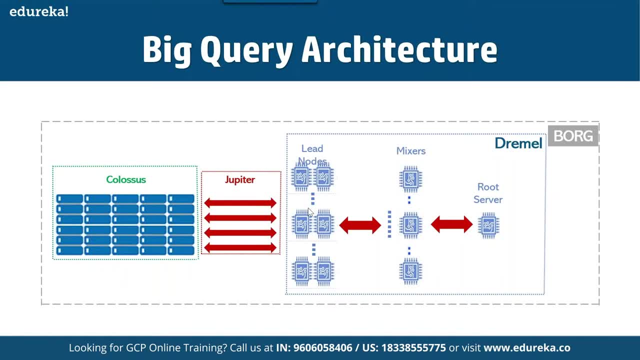 multiple nodes connected. you know where you're going to have: the entire leaves and mixture. so we are going to have the uh, the topmost hierarchy, which is known as root, then you are going to have which is known as mixers and at the end you are going to have the lead nodes, which is going to 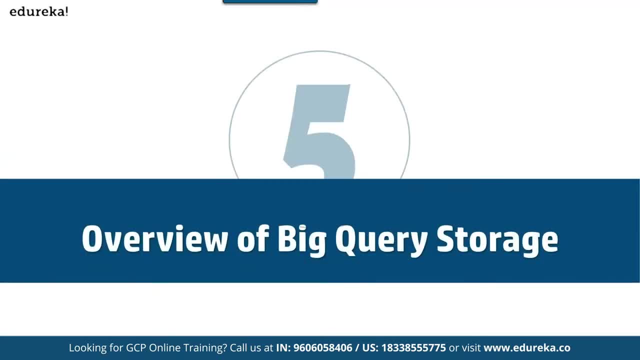 you know, communicate with your colossus talking about here big query storage. so basically, in the case of big query storage, you have different type of storage management. so primarily you are going to have two different type of storages. the first storage is basically your traditional storage. 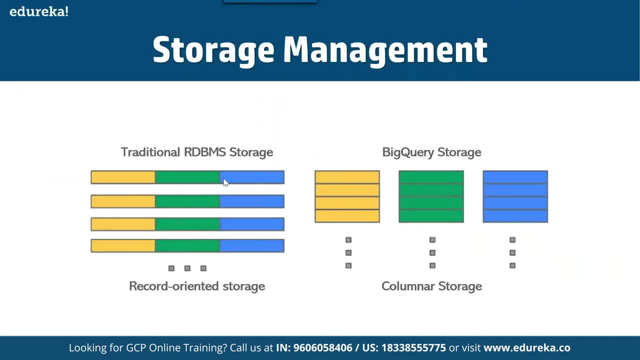 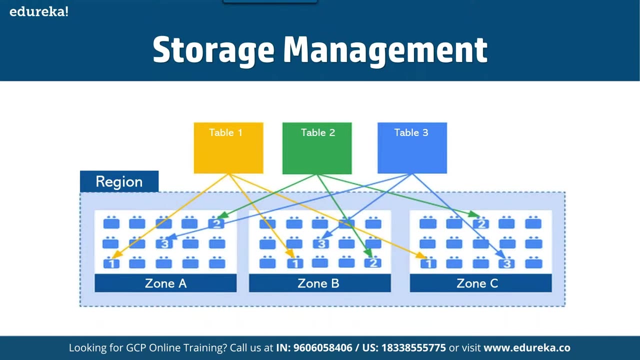 which is known as record oriented storage, which is basically row wise. next is your big query storage, which is basically nothing, just a column level storage that you have now. this is basically your table: one table, two tables with different tables. you have different zones. you have you can put and segregate your data with. 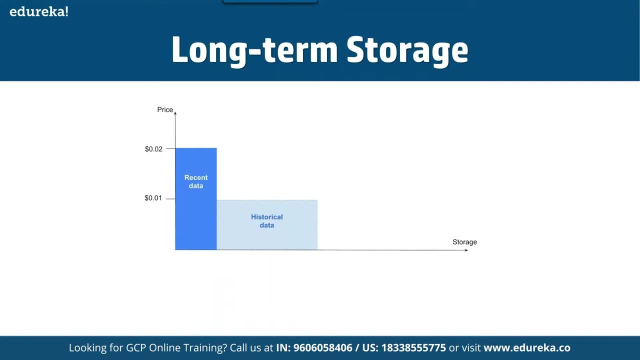 each other. now we have a concept of lts, which is long term storage. so if you have a table or partition which is not not modified for 90 consecutive days, it is considered long term storage and the price of storage for that table automatically drops by 50 to the same cost as. 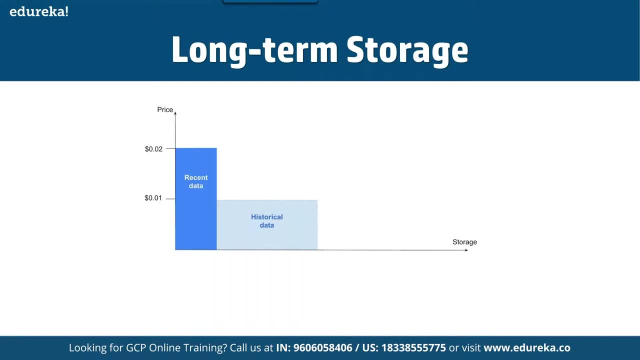 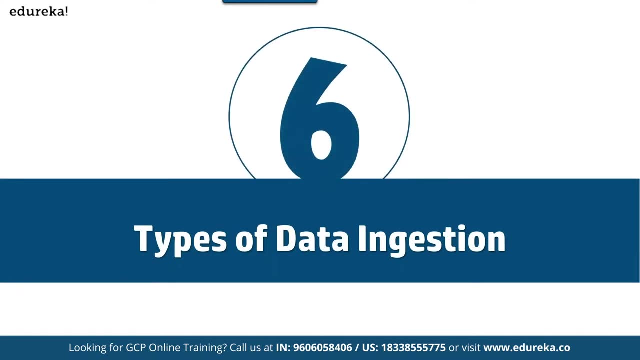 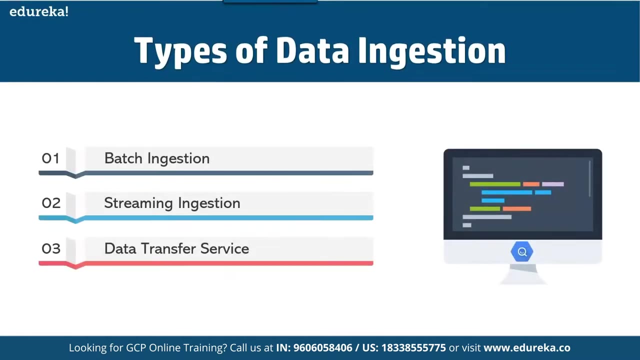 cloud storage nearline, so discount is basically applied on per table, per partition basis. now you have three types of data ingestion available. one is batch ingestion, second is streaming ingestion and third is data transfer service. talking about each of this category, the fold, which is your batch injection. 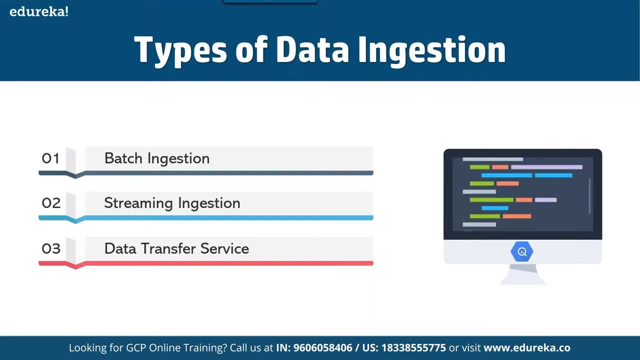 batch ingestion involves, you know, you know- loading your large bounded data set that don't have to be processed in the real time. they are typically ingested at a content called the tf mestasrart, which is the holistic categorization system that allows you to be redistributed to all your storage. 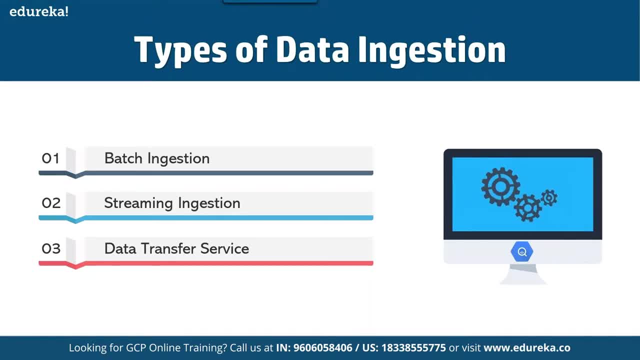 material in a civilizations locally referred to as the operating platform and verse the sales chart. Now talk to me about this. I'll let you move to the description of Mirovets. specific, regular frequencies and all the data arise at once and not at all. So the ingested 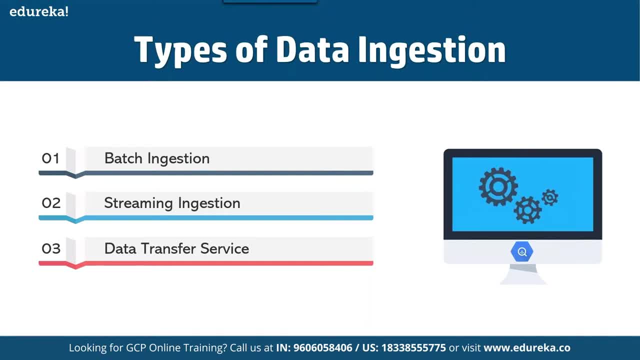 data is then queried for creating reports or combined with other sources, including real-time data that we have. Next one that we have is a streaming ingestion. In the case of streaming ingestion, you're going to inject the data from various sources in the form of pipeline. 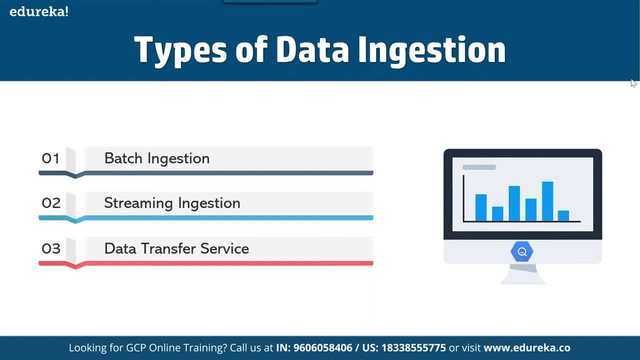 and once we have the data available, you are going to link that data and you're going to work on that data all together. And last one that you have is the third one, which is DTS, which is known as data transfer service. So the BigQuery data transfer service is a fully managed service to ingest data. 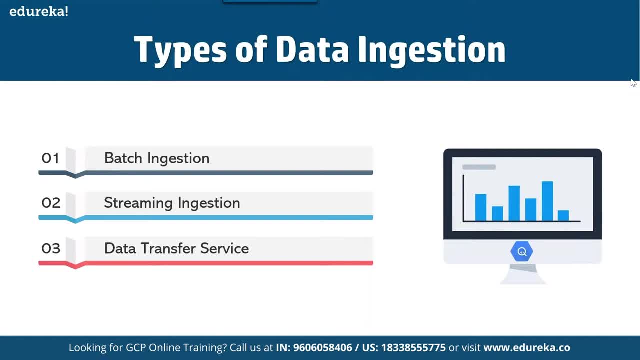 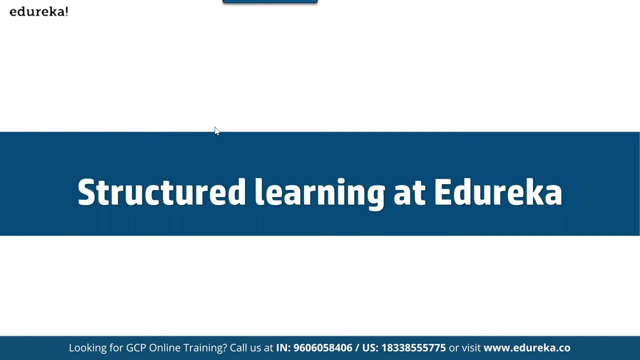 from Google software service application like Google Ads. external cloud storage providers like Amazon S3, transferring data from data warehouse technologies such as DataRadar, Amazon Redshift. Now talking about your structured learning at Edureka: If you are highly interested to learn the course, you can go to edurekacom. You can also go to edurekacom If you are highly. 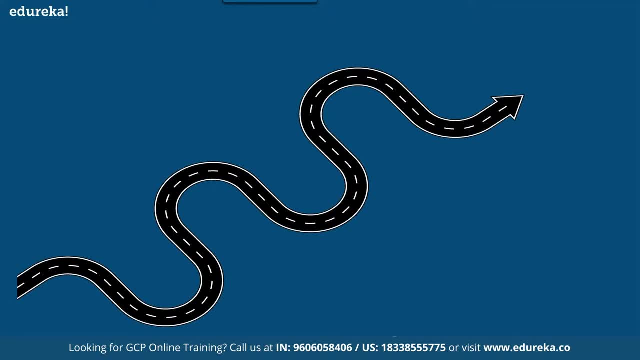 interested to learn the course, you can go to edurekacom. You can also go to edurekacom. If you are highly interested to learn the course, you can go to edurekacom. So these are some of the resources into and in detail, how your journey is going to look like. what are all the topics we are going? 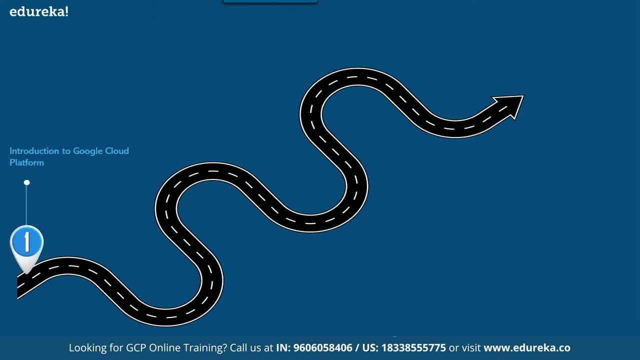 to cover. Let's talk about it. In the very first class, you're going to learn about Google cloud platform. What is google cloud platform? what are the components of it? So all the basic things in detail. you are going to learn with the practical, hands-on Post that in the second class you will 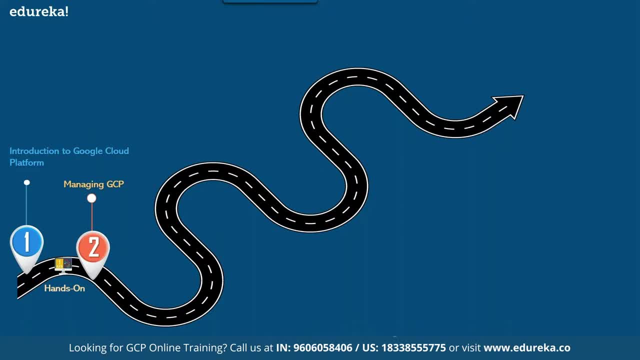 learn about how to manage the GCP, How to basically manage the Google cloud platform, with the practical hands-on. Suppose that in the third class you will learn about the Google Cloud platform, the virtual networks and everything with the practical hands-on. Then in the fourth class, 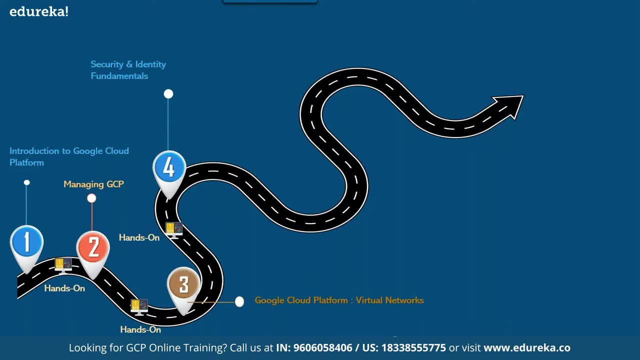 you will learn about security and identity- fundamentals with the practical hands-on In the fifth class. you will learn about compute service: the different type of compute services that you have being available, on which you can work on with the practical hands-on In the sixth. 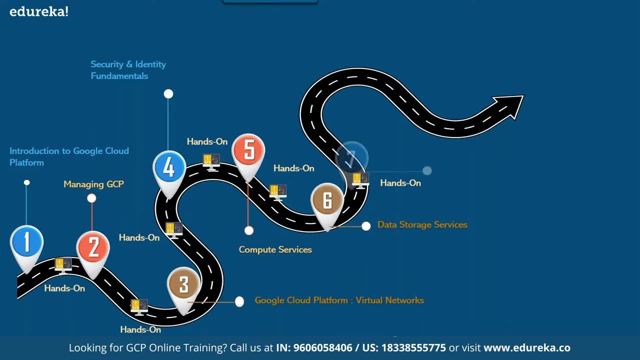 class, you will learn about DSS, which is data storage services, with the hands-on. In the seventh class, you will learn about architecting with Google Kubernetes engine with the hands-on. In the eighth class, you will learn about application development with the hands-on.